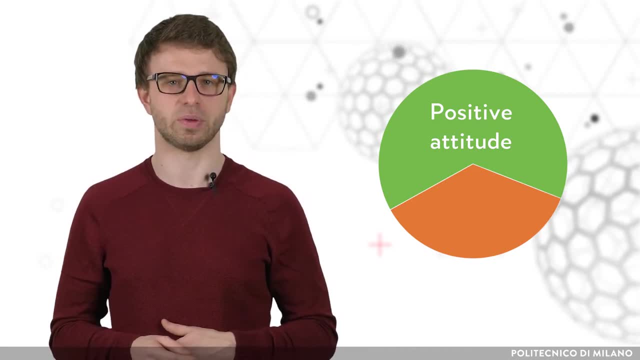 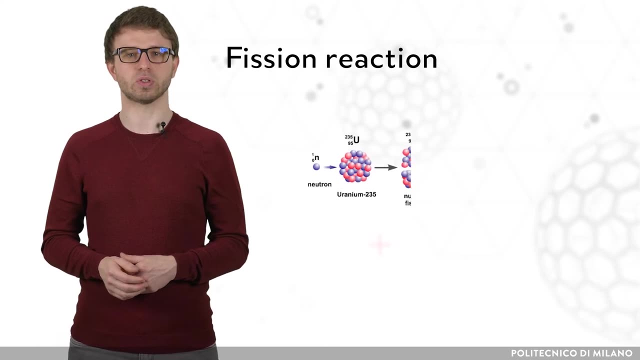 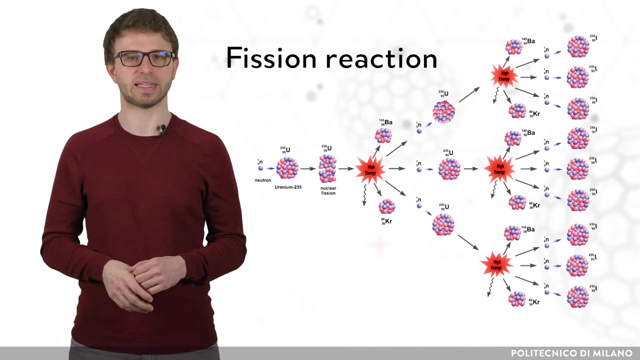 less greenhouse gases than, for instance, fossil fuels. To produce energy, nuclear reactors exploit fission reactions induced by neutrons or nuclear fuel containing fissile isotopes. If these reactions are able to produce more neutrons, it is then possible to sustain a fission chain reaction. 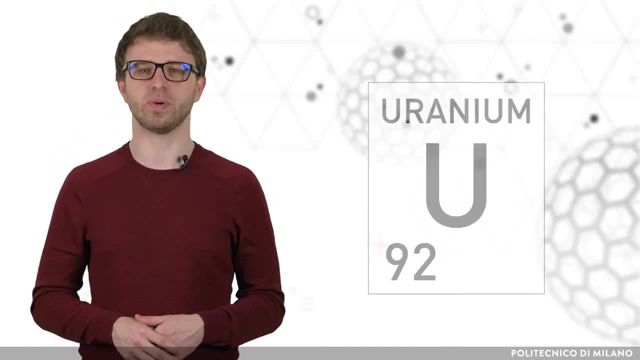 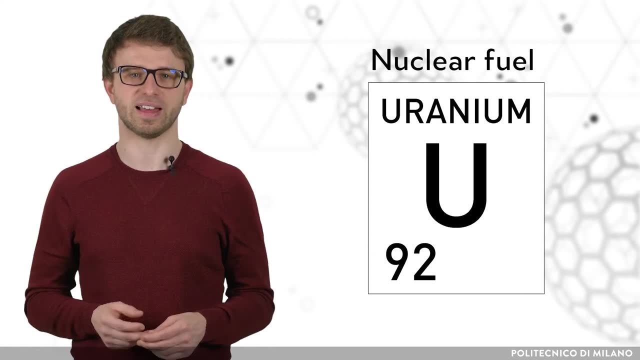 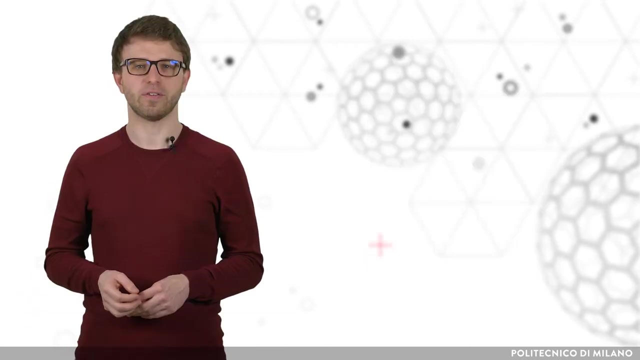 Nuclear fuel consists of uranium oxide, which is often enriched in the fissile isotope uranium-235.. Uranium is extracted from uranium ore and fuel is produced in dedicated fuel fabrication plants. After use in a nuclear power plant, the composition of the fuel is changed due to nuclear reactions. 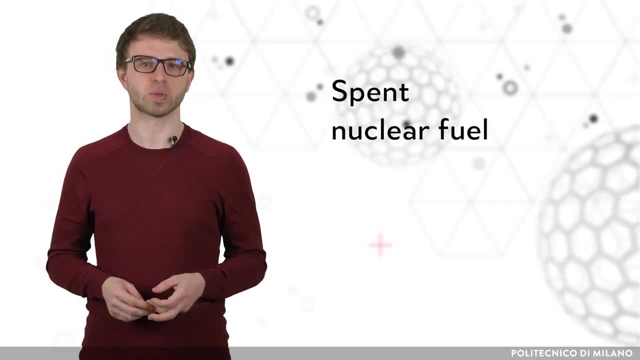 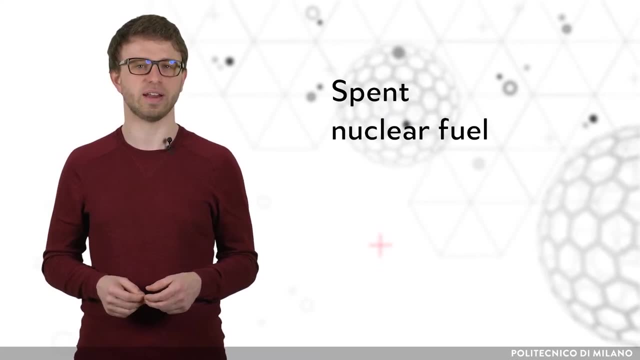 When discharged from the reactor, it is called spenuclear fuel. This needs to be further managed. It is worth noting that only a small fraction of the energy available from fission of the nuclear fuel has been consumed. By the time the fission of the nuclear fuel has been consumed, the energy 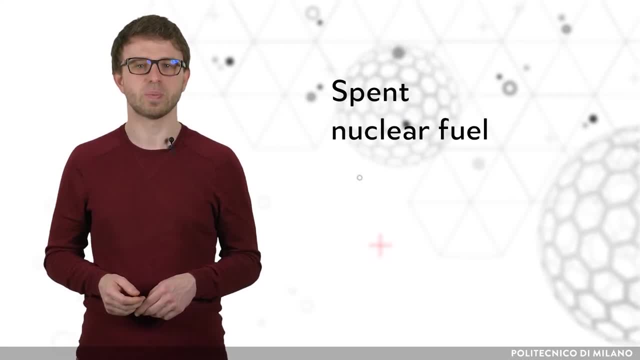 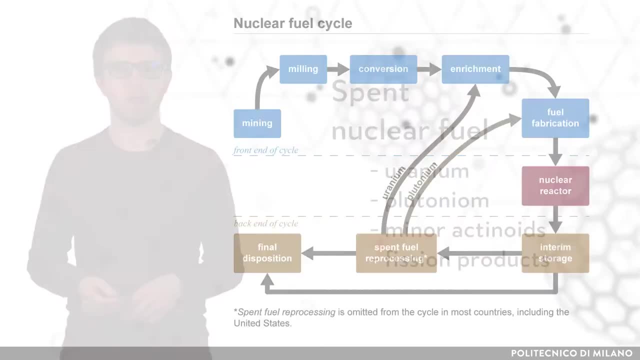 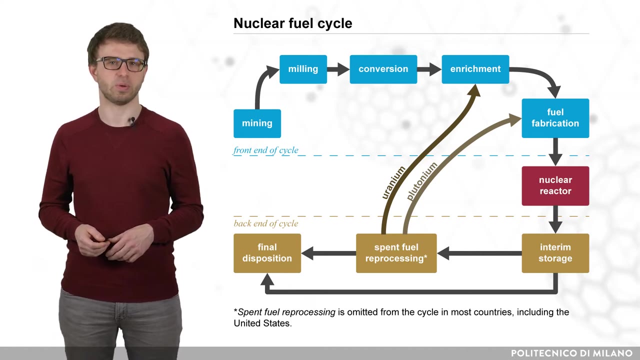 the fuel is discharged from the reactor. Spent nuclear fuel consists of uranium, plutonium, minor actinoids and fission products. All of these steps constitute the nuclear fuel cycle. In particular, uranium mining, uranium enrichment and fuel fabrication are generally indicated. 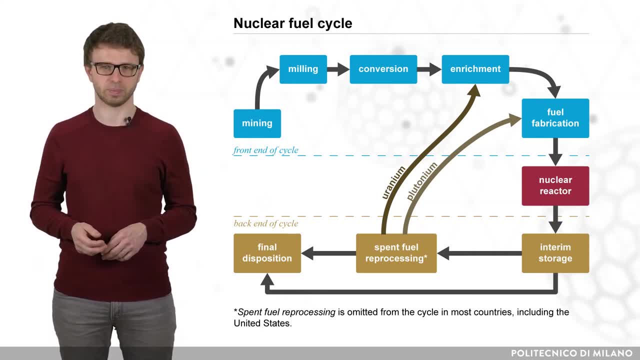 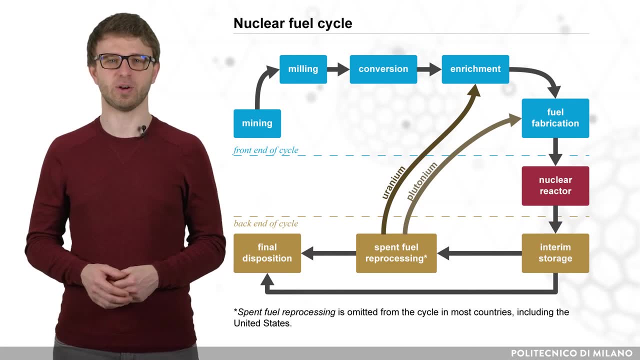 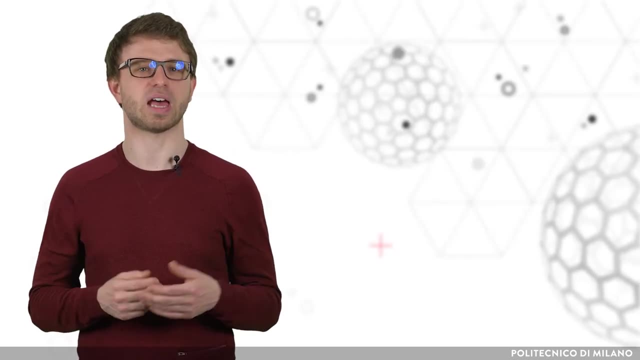 as the front end of the nuclear fuel cycle. After discharge from the reactor, in the so-called back end of the nuclear fuel cycle, there may be different options after the spent fuel has cooled for a suitable period of time. There are two main scenarios how to deal with spent nuclear fuel. 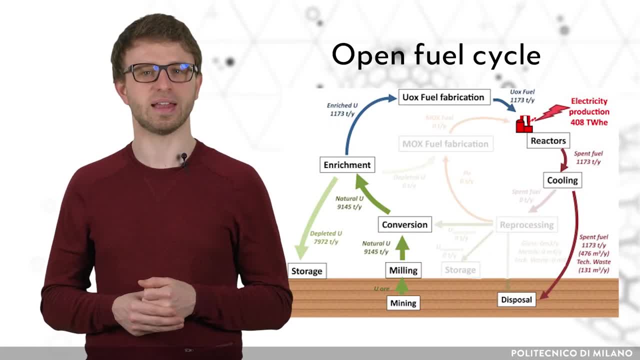 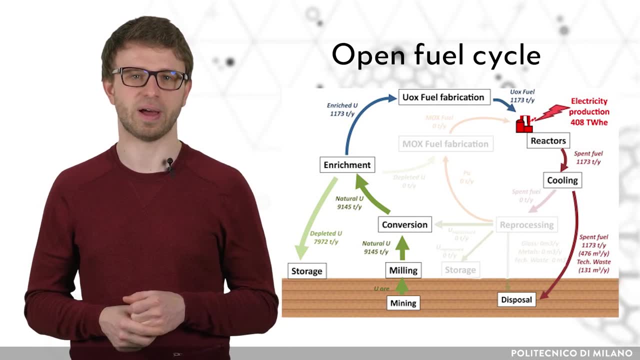 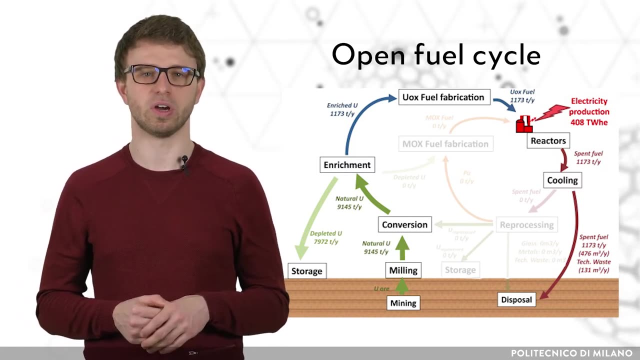 Spent nuclear fuel can be considered as waste and disposed of into deep underground repositories. Such waste is characterized by a significant volume and long-term radiotoxicity. Furthermore, it still contains much of the originally present uranium and also plutonium produced during irradiation. 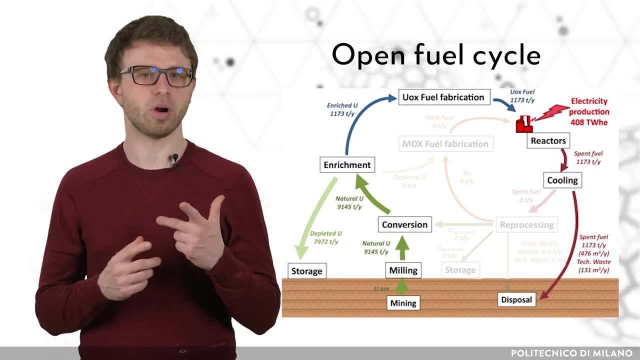 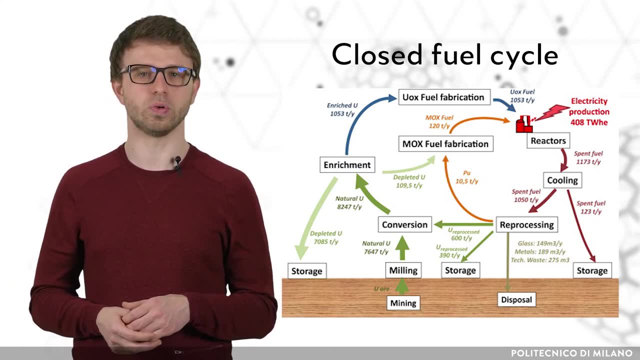 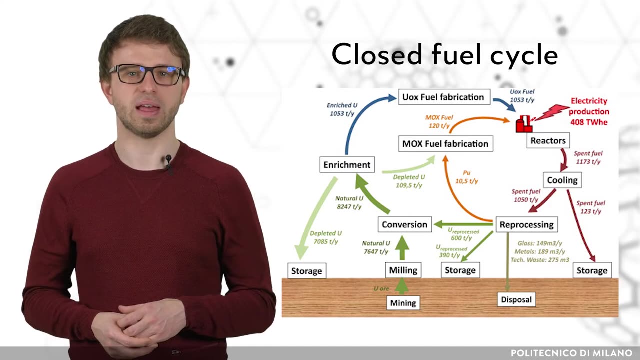 This option is called the open cycle. In a more sustainable view, these valuable elements could be separated from fission products and used to produce new fuel make of mixed uranium and plutonium oxides. The second scenario, the so-called closed fuel cycle. 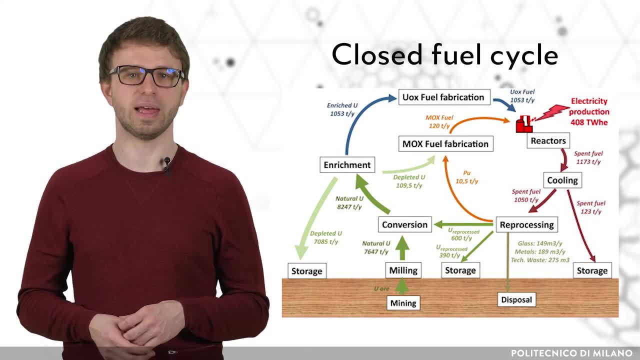 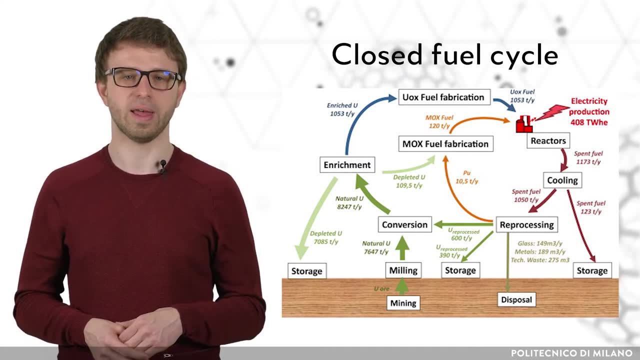 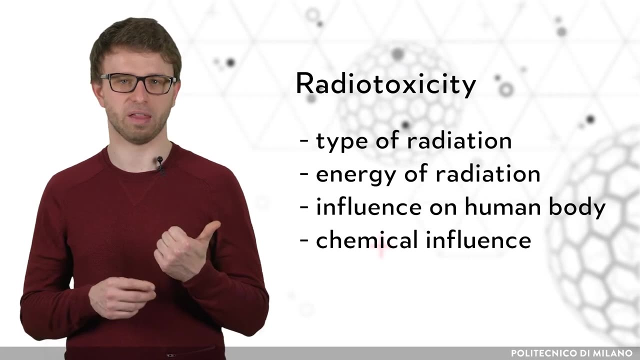 is based on reprocessing of spent nuclear fuel, leading not only to uranium recycling but also to a reduction of the overall waste volume and radiotoxicity. Radiotoxicity considers the type of radiation- alpha, beta, gamma or neutrons- and its energy. 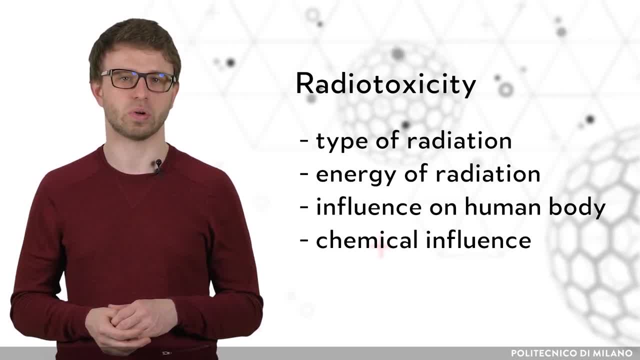 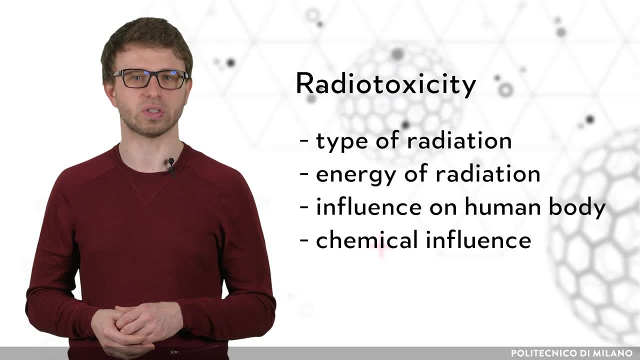 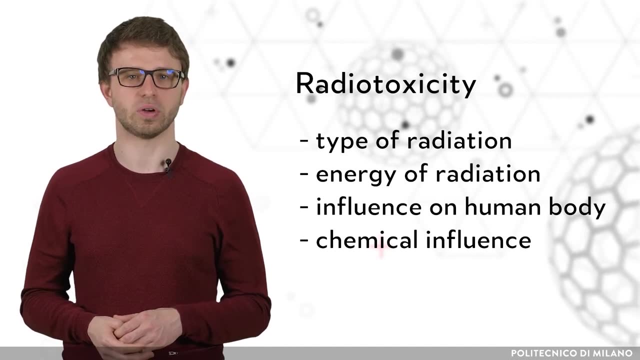 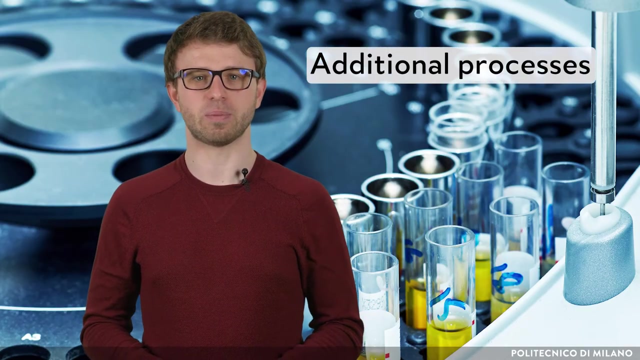 influence on the human body as the dose conversion factor, and chemical influences on living tissues. Therefore, radiotoxicity is an important parameter for consideration in the nuclear fuel cycle, which is based on the particular isotopes present in spent nuclear fuel After the reprocessing, the volume and long-term radiotoxicity of the reprocessed waste can. 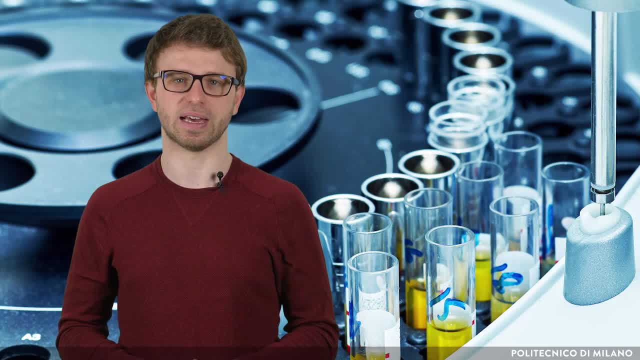 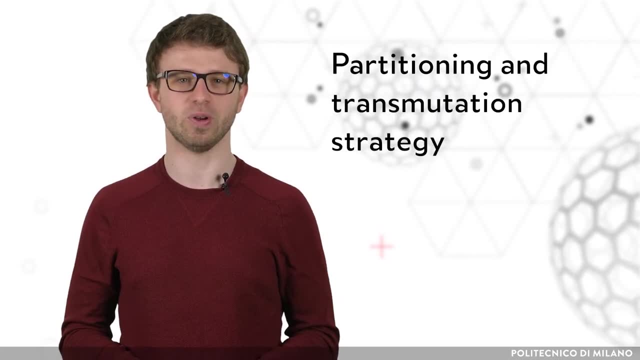 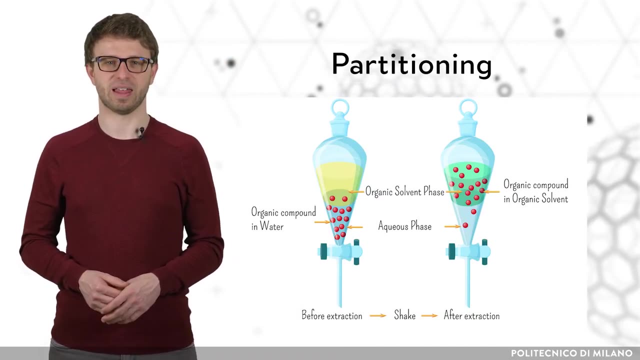 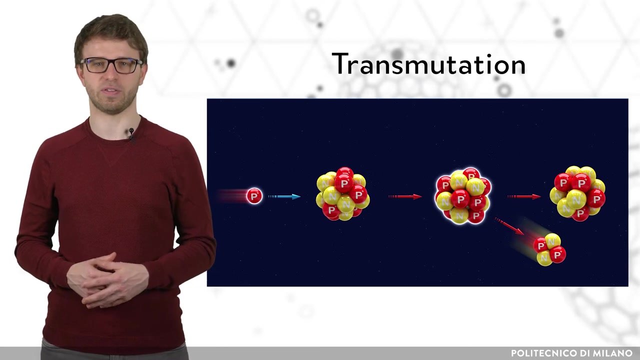 be further reduced by additional chemical processing, sometimes called partitioning. Research related to the advanced reprocessing of spent nuclear fuel has shown that radio-toxicity can be measured in the same way as an behaviors of the. from said radio-toxicity, The onset of the Recent Recoffer is accelerated tonautical. 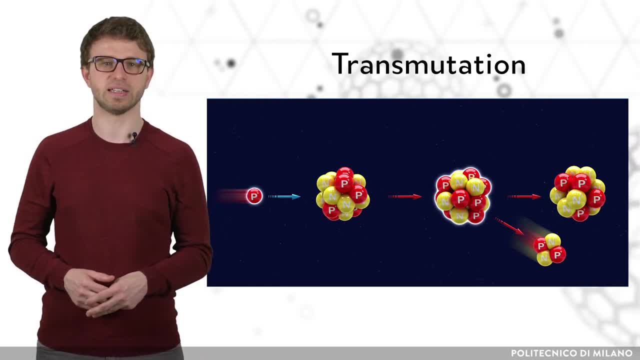 from the carbon dioxide layer and is called partitioning and transmutation. Partitioning processes aim to separate the long lived elements, such as some actinides. The subsequent transmutation refers to the conversion of the separated long-lived radionuclides to short lived radionuclides or stable elements by nuclear reactions, eg in dedicated accelerator-driven. 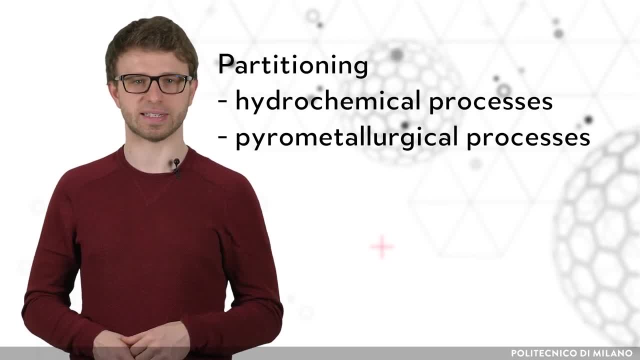 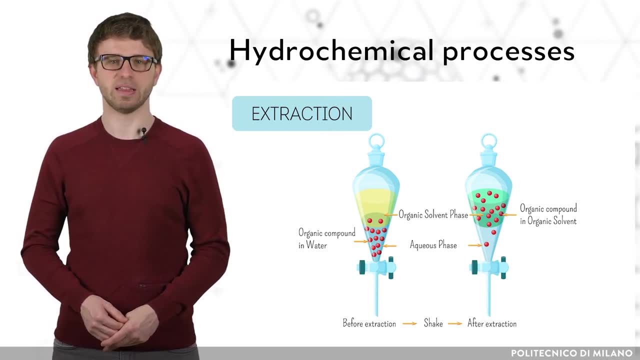 transmuters. Partitioning can be based on either hydrochemical or partitioning pyrometallurgical processes. In hydrochemical processes, spent nuclear fuel is firstly dissolved in nitric acid. The following processes are mainly based on solvent extraction technique due to the application. 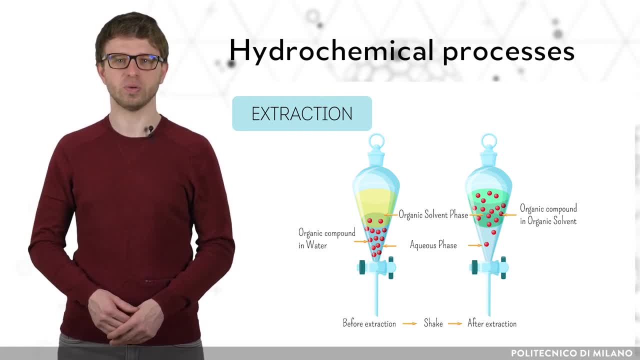 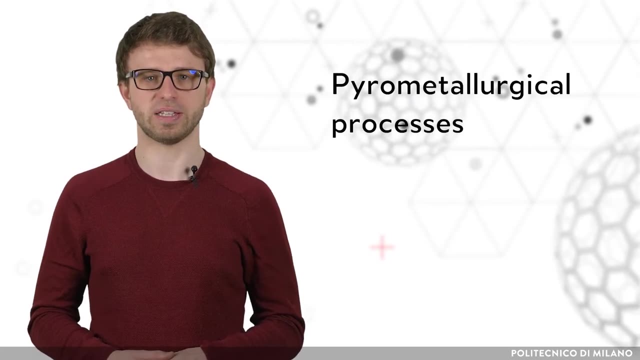 of citable extractin ligands in solution. Those extractin ligands transfer the radionuclides between two phases and separate them. There are many different steps to separate all of the desired elements. Pyrometallurgical processes exploit high temperatures and has the advantage of being. 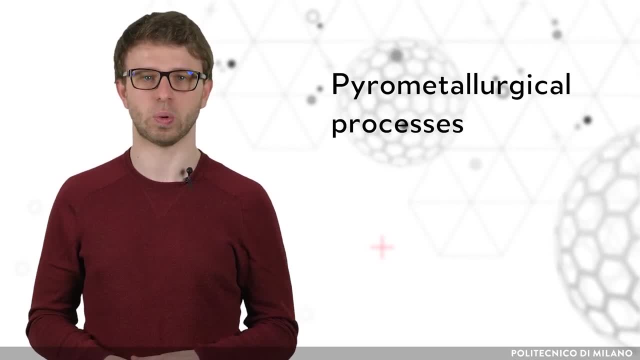 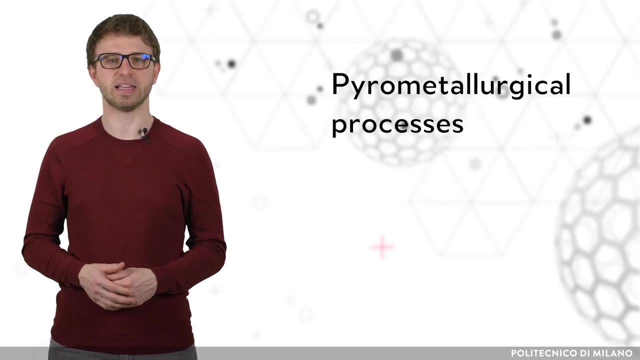 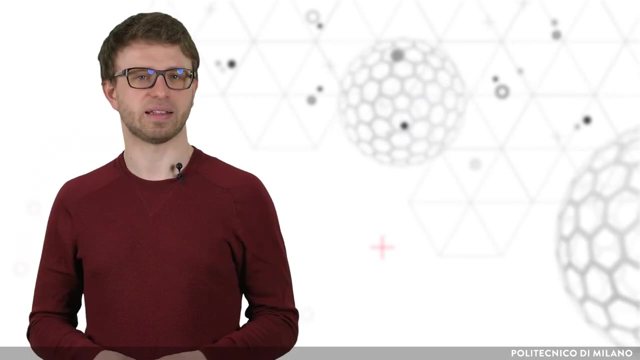 able to treat spent nuclear fuel after a shorter cooling time. In these processes the spent fuel is melted and the melt is processed, eg electrochemically or by liquid-liquid extraction, where the fluids are liquid metals. Currently, the only process operated routinely on an industrial scale is the hydrochemical.